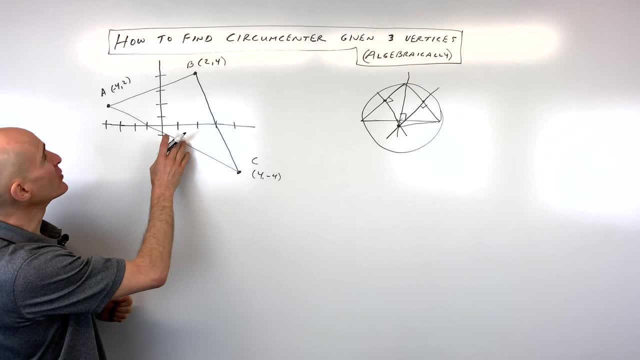 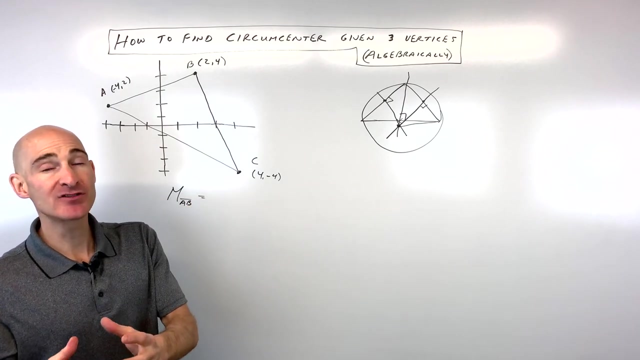 the circle here. So let's go ahead and jump into this particular example here. The first thing I want to do is I want to find the midpoint of side AB, So I'm just going to denote that as segment AB. Now, when you find the midpoint, what you want to do is you want to find the average of 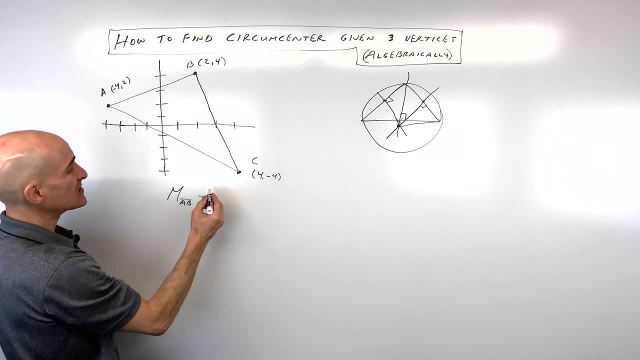 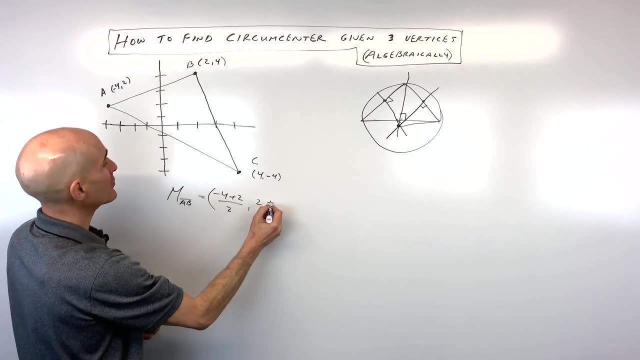 the x's and the average of the y's. So what we do is we add the x's together, negative four plus two, and we divide by two. Same thing with the y coordinates: We take the y's, we add them together. 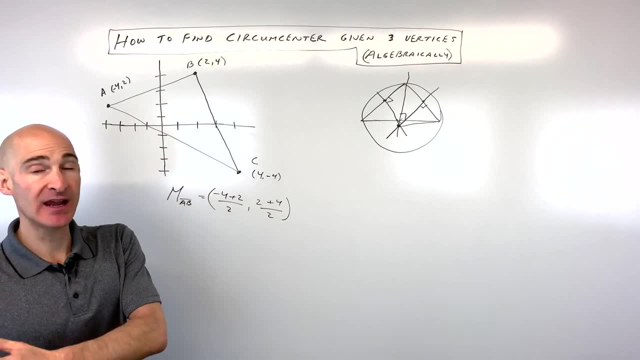 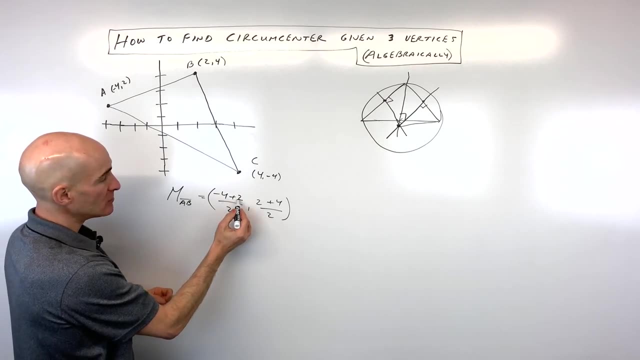 two plus four and we divide by two. So just think of like an average, like if you get an 80% and 100%. you add those together, divide by two. that's going to be your average, right? So here we've got negative two divided by two, which is negative one. Two plus four is six. 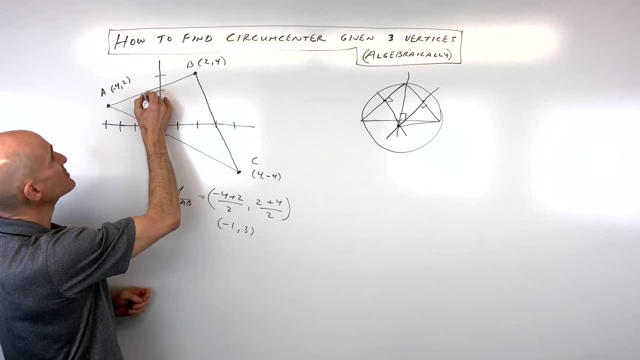 is three. So the midpoint here should be at negative one, positive three. okay, Now my drawing's. you know a little bit off, I just did this freehand, but that's going to be the midpoint here. Now, what we want to do is we want to find the perpendicular to this side AB. So we have to. 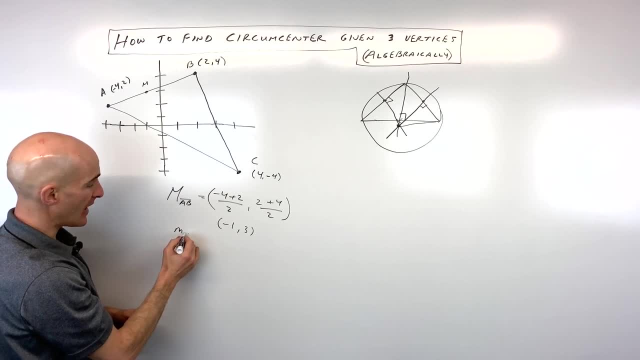 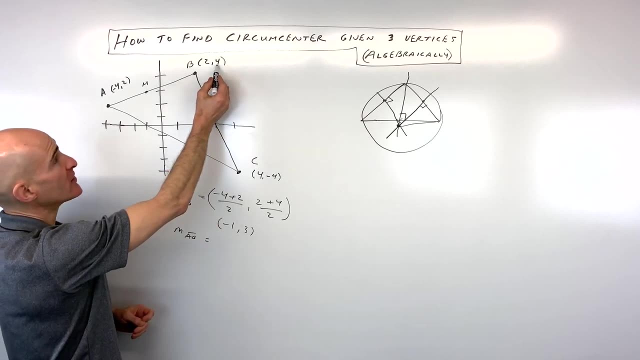 find the slope of AB. So I'm going to denote that with a lowercase m for slope, So the slope of side AB. And to find the slope, we do the y2 minus y1 over x2 minus x1, the slope formula. So we do four. 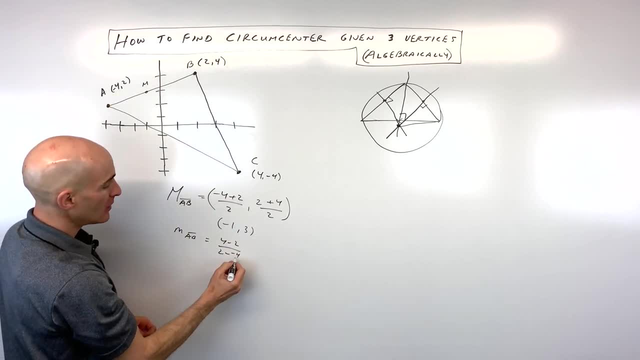 over two minus negative four. Remember, when you subtract it's like adding the opposite. So this is going to give us two, six, which is one third Now if we find the perpendicular, okay. so I denoted that with the perpendicular symbol we have to take the opposite reciprocal. So I'm going 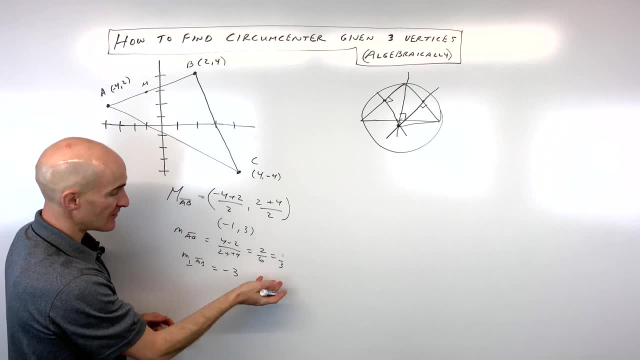 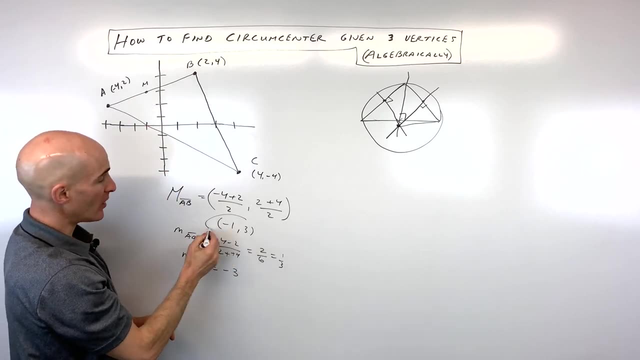 to change this to negative. since this is positive, I'm going to flip it over. that's going to give us negative three. So we know that the slope is negative three and it goes through the midpoint here, which is negative one three. So if we put that together, we're going to get negative three. 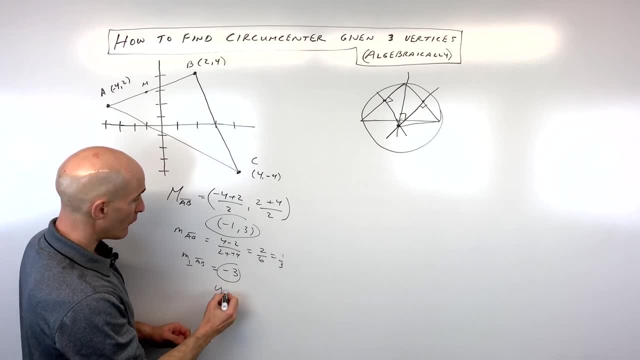 So if we put that together into an equation using the point slope formula, we have y minus three. So y minus the y coordinate equals the slope which is negative three times x minus the x coordinate. Well, x minus a negative one is like x plus one. Now I can simplify this a little bit. 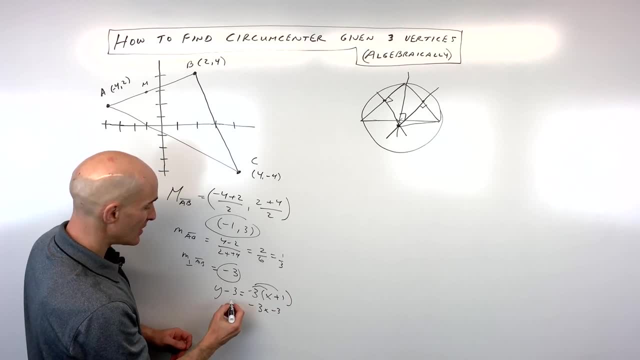 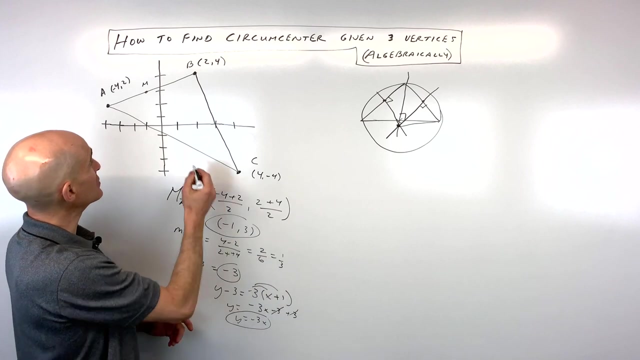 further by distributing, That gives us negative three x minus three. And if I add three, this three over here to both sides, that's going to give us y equals negative three x, the negative three and the positive three cancel. So we're getting y equals negative three x. So what that means is the y intercept is zero, it's going. 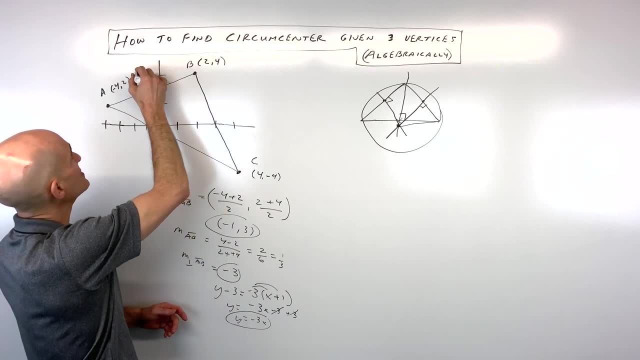 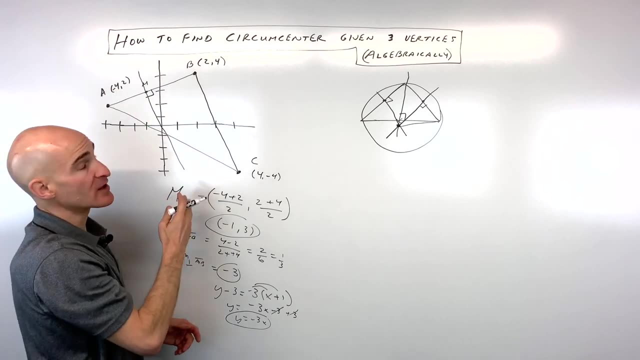 right here through the origin. So the line is going to look something like this: Okay, I'm just rough sketching right here. Okay, so that's the equation of one of the perpendicular bisectors. So bisected, cut that in half and it was perpendicular. Okay, so now what we need to do is: 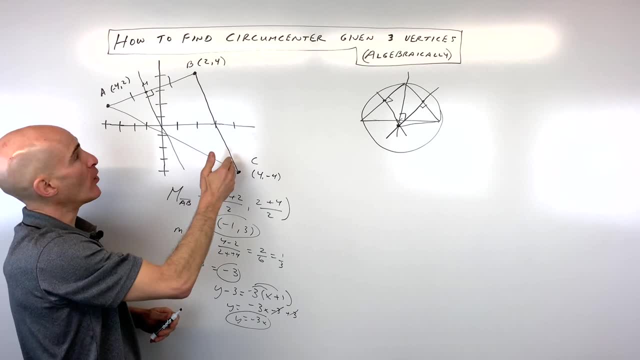 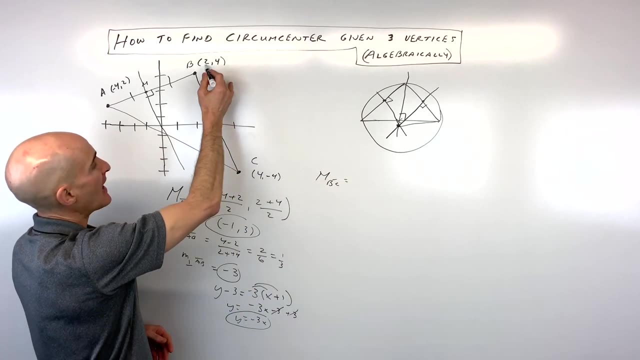 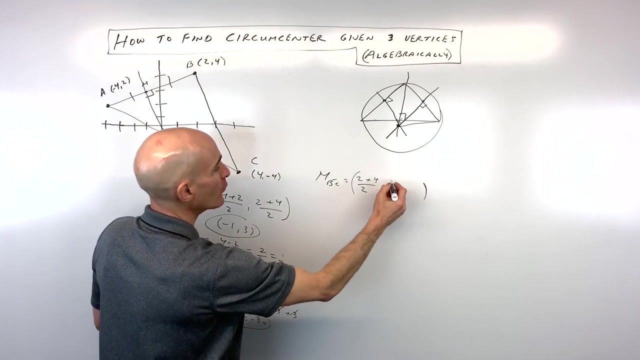 find the slope and the midpoint of this side, bc. So let's go ahead and find the midpoint first. So, bc, we're going to take the average of the axis, so two plus four divided by two, and we're going to take the average of the y's, four plus negative four divided by two. So that slope, I'm sorry not. 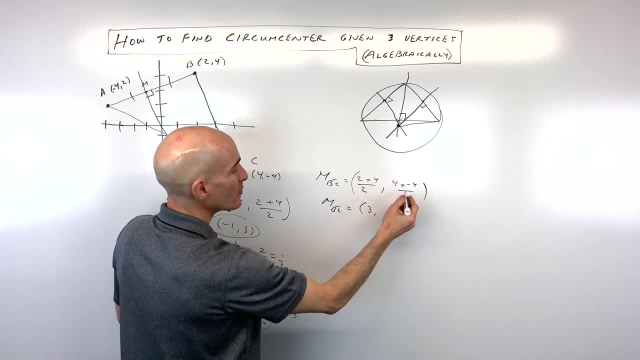 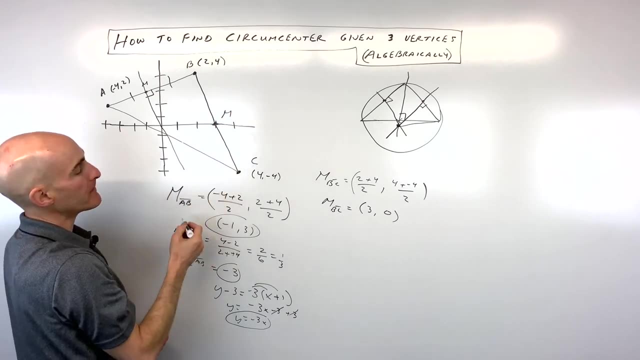 that slope. but the midpoint comes out to six over two, which is three. Four plus negative four is zero over two, which is zero. So it looks like the midpoint is going to be here at three comma zero. Okay, so midpoint: We want to find the slope of bc, so we're going to use our slope formula. So. 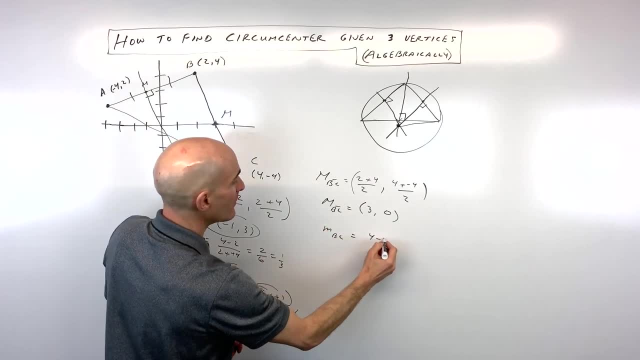 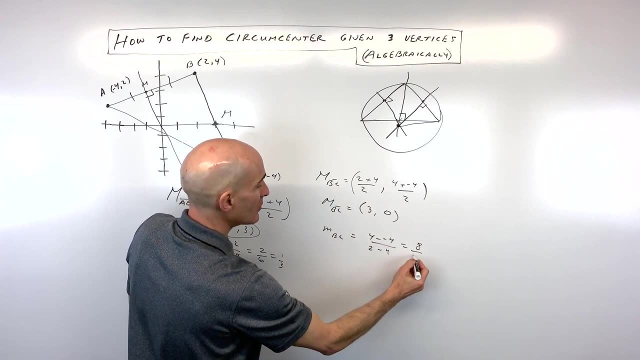 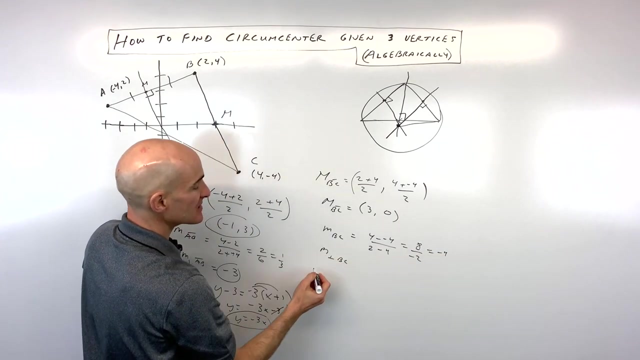 bc that equals y two minus y one, so four minus negative four over x two minus x one, so two minus four. So that comes out to eight over negative two, which is negative four. But the slope of the perpendicular to bc is going to be the opposite reciprocal, So I'm going to flip that over and 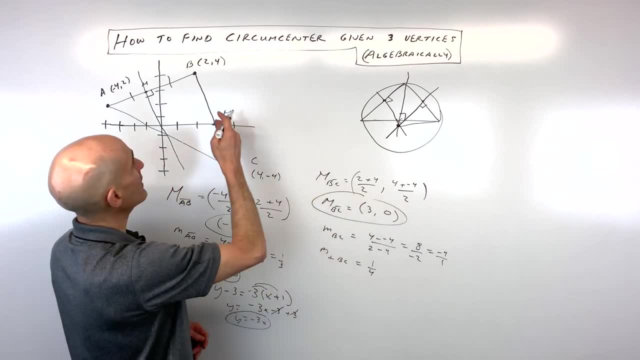 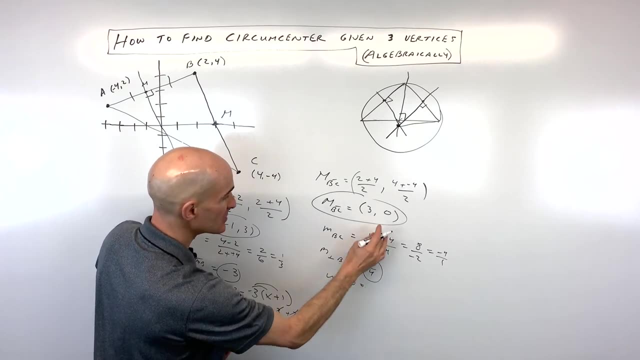 change the sign, so it's going to be one fourth. So if we take the point three, zero and a slope of one fourth, put that together using our point slope form, this is going to be: y minus the y coordinate equals the slope times x minus the x. 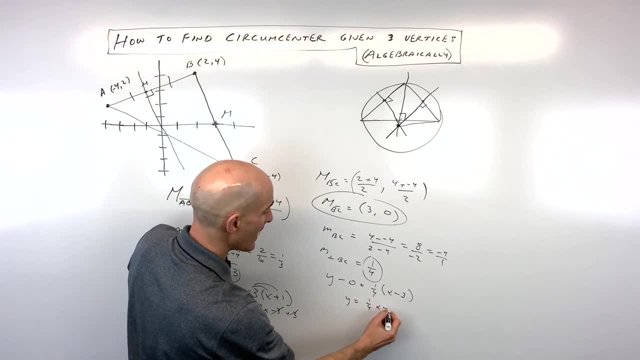 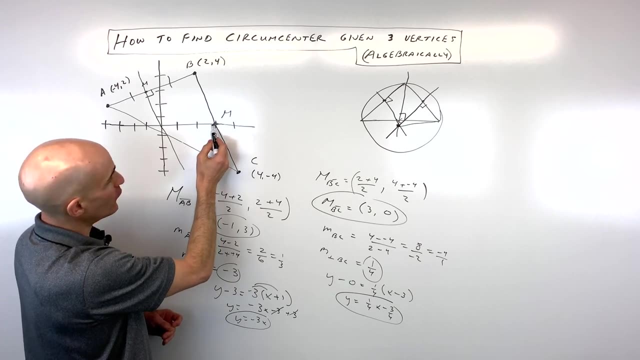 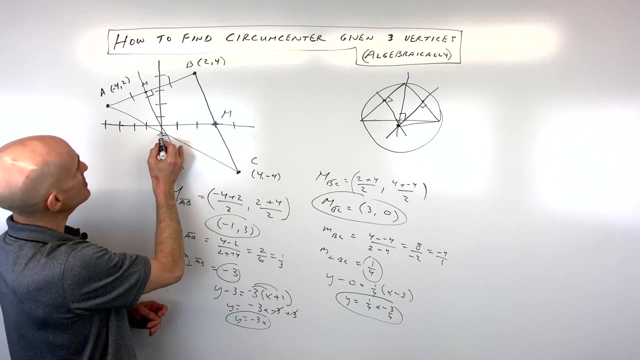 coordinate, We get: y equals one fourth, x minus three fourths. So now let's go ahead and draw that line in here. So this is going to be a slope of negative three fourths. So that's going to be- let's see, y intercept of negative three fourths is somewhere right around here And a slope of. 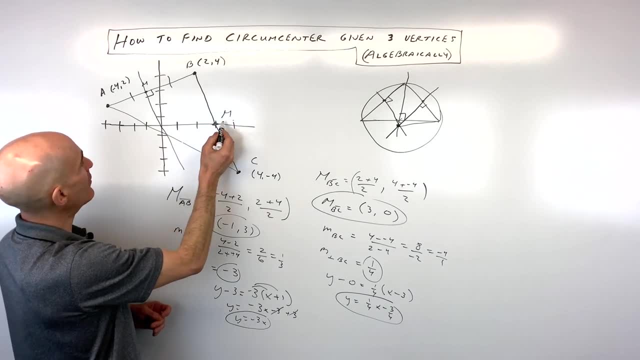 rise one, run four, something around here. So that's going to be a slope of negative three here. So it looks like it's going to go something like that. Okay, so it looks like they're crossing right here, But let's use the algebra to find that common point of intersection. So we're going to. 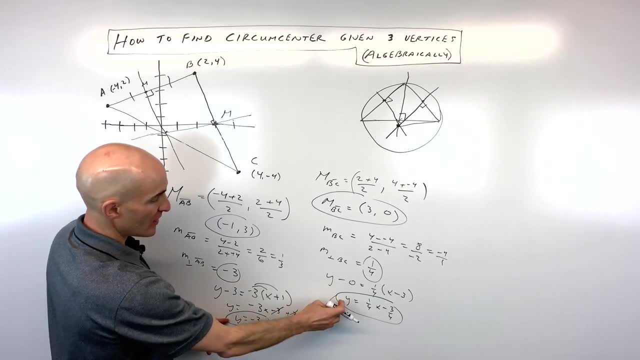 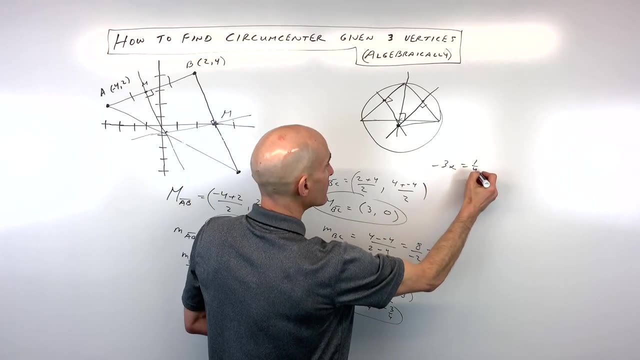 go ahead and do a substitution. If y equals negative three x, I'm going to put negative three x in place of y. So let me write that over here. So negative three x equals one fourth x minus three fourths. Now here's the thing: a lot of times when students get a lot of fractions, 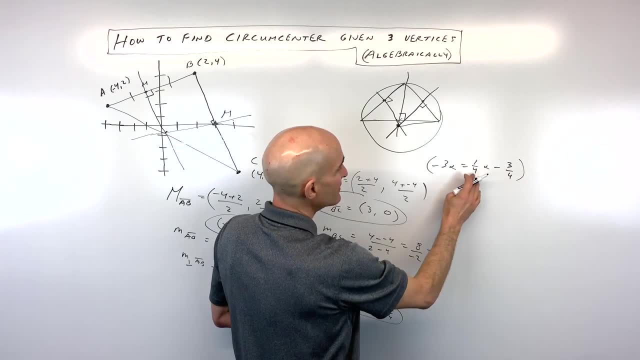 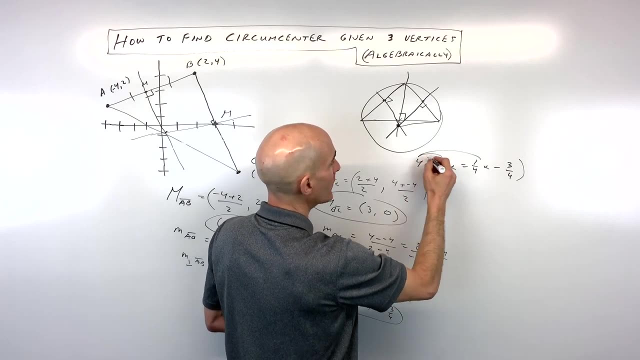 you know they get a little bit intimidated. But since we have common denominator of four, like like: this is over one, four, four, four is like our common denominator- I'm going to multiply everything by four to clear the fractions. So four times. 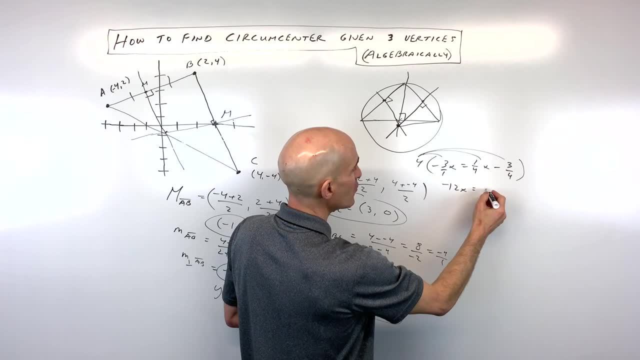 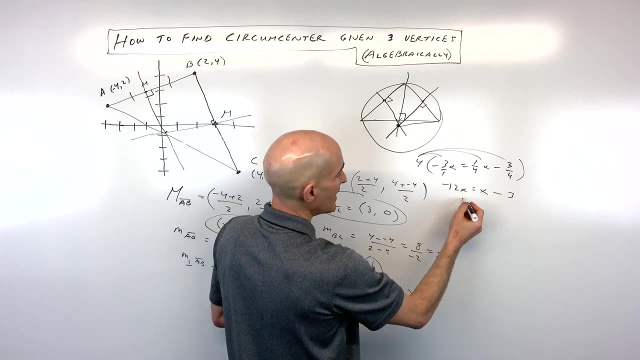 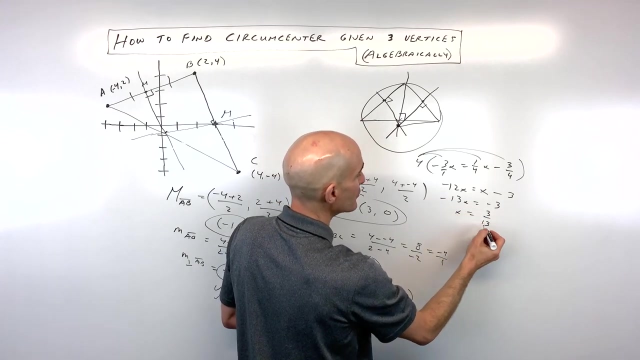 negative three gives us negative 12x four times one. fourth is one, so that's just x. And then these fours are going to cancel. that just gives us minus three. So if I subtract x from both sides, I get negative 13x equals negative three. divide both sides by negative 13x equals three thirteenths. 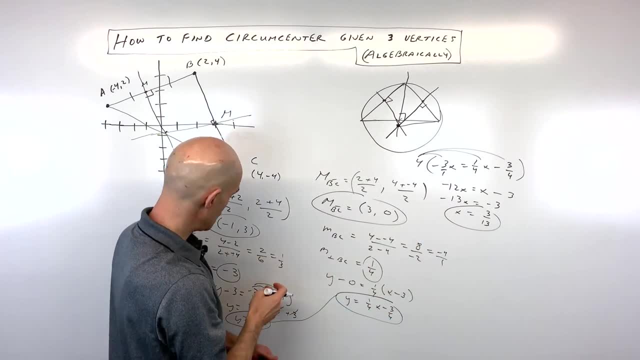 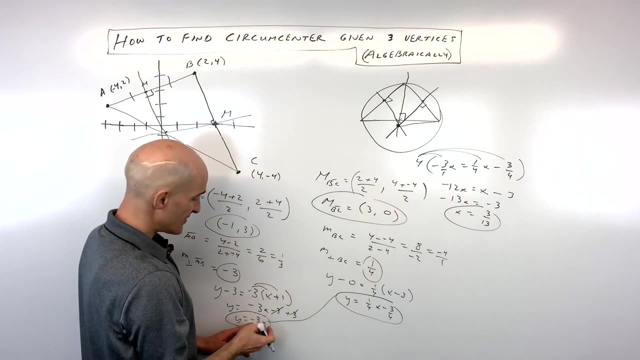 If I take three thirteenths and I put it back in either into this equation or this equation, I'll do this one, since it's a little bit easier. Negative three times three thirteenths gives us negative nine thirteenths. 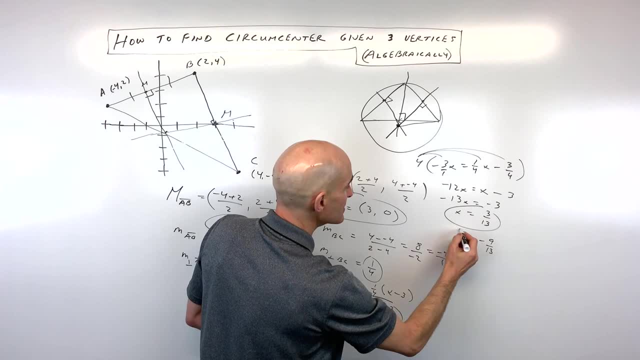 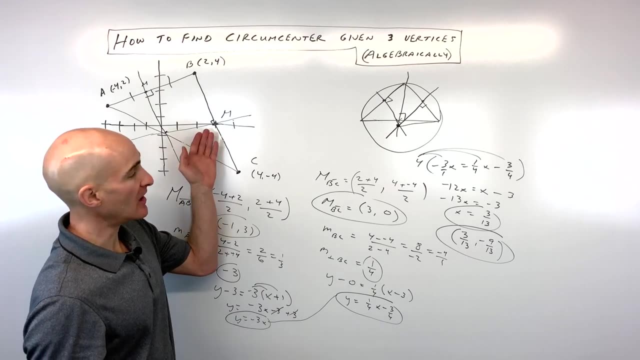 So three thirteenths, comma negative nine thirteenths. that's going to be our common point of intersection of our two perpendicular bisectors and that's going to be our circumcenter. So let's see if that's accurate. here We've got three thirteenths, okay, negative nine thirteenths. 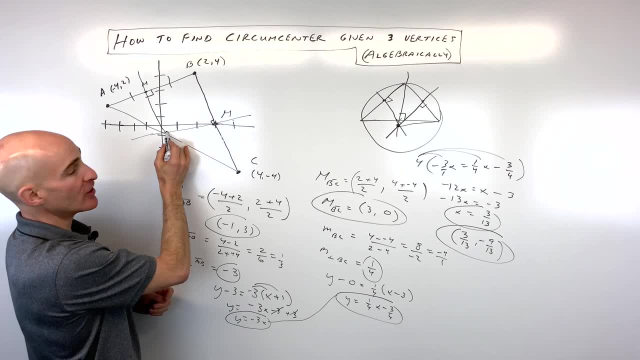 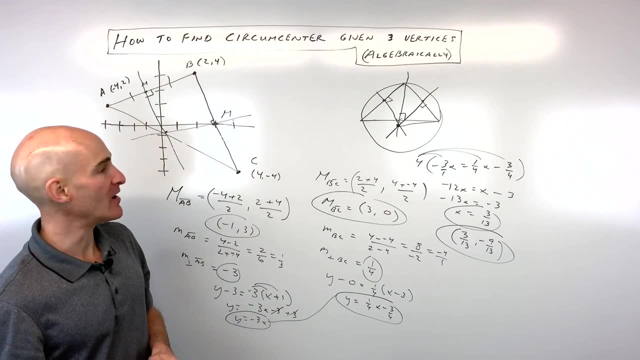 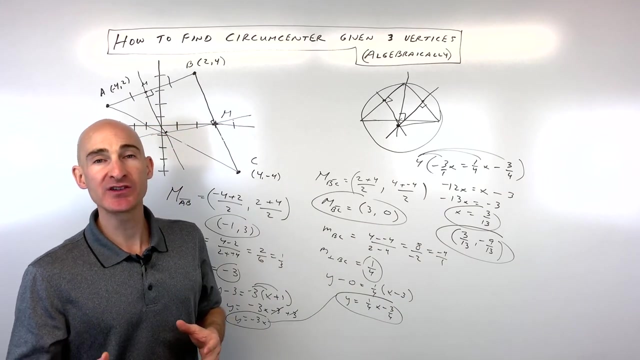 pretty, pretty good, you know pretty close. Okay, my diagram is a little bit off because the spacing of the x and y scale are not exactly perfect like on graph paper, right? But that's how you would do it algebraically. So if you want to see how to do this using constructions with a compass and a, 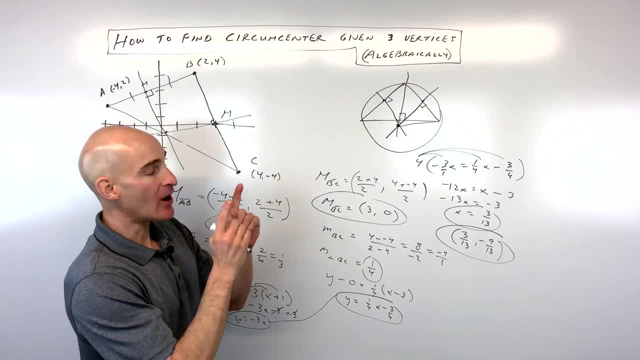 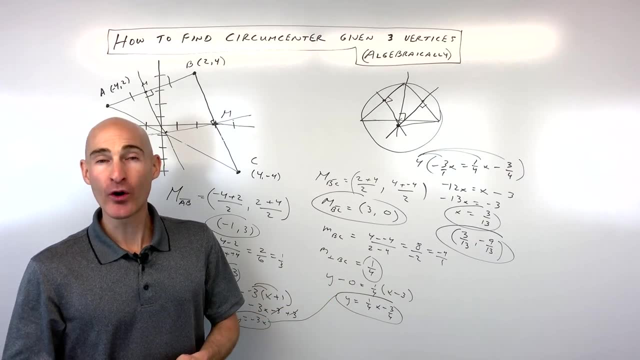 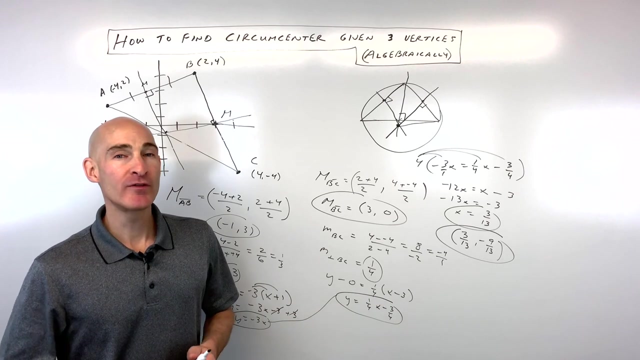 protractor and a straight edge and all that. go ahead and check out the video I did right there, Great job. If you like the way that I teach and you're interested in learning more about algebra, geometry, algebra two, precalculus, ACT math, SAT math, check out more videos. 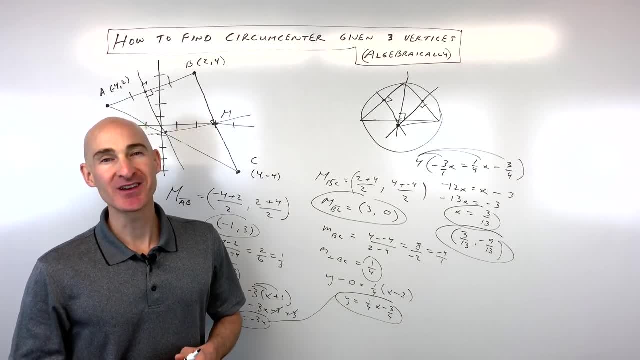 on my Mario's Math Tutoring YouTube channel and I'll see you in the other videos. I'll talk to you then.